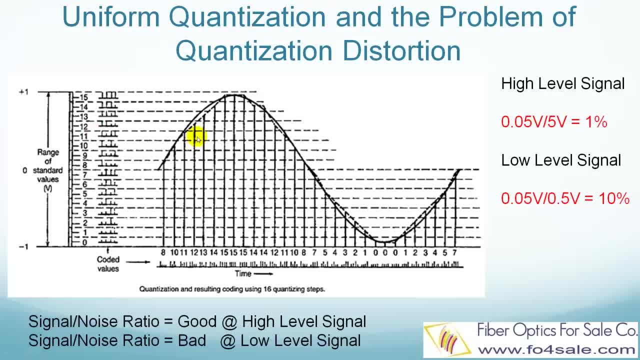 The range between 1 volt and minus 1 volt is divided into 16 steps. Each step represents 0.125 volt. Forémult samples whose amplitude falls within a step take the same step value. However, the quantization process introduces an error. 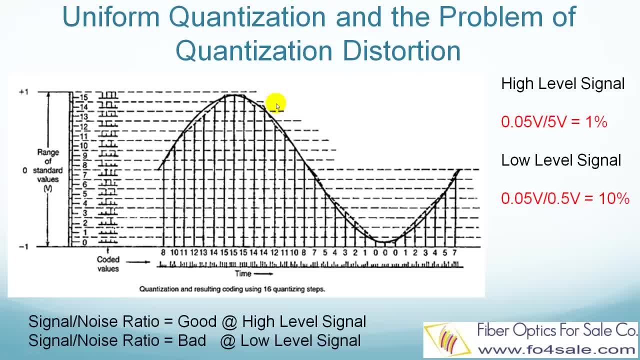 This is because that the real amplitude of a sample is replaced by the approximate value. This error is called quantization noise or quantization distortion. In uniform quantization, the quantization distortion presents a problem, For example. For example, let's assume a quantization error of 0.05V. 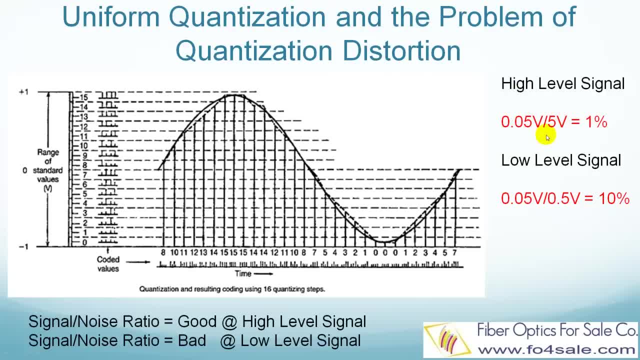 If this happens at a high-level signal, such as 5V, the noise ratio is 0.05V divided by 5V, which is 1%. not too bad. But if the same quantization error happens at a low-level signal, such as 0.5V, the noise 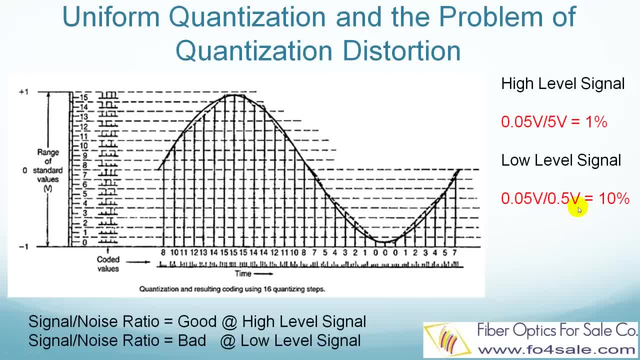 ratio is 0.05V divided by 0.5V, which is 10%. Simply put, for uniform quantization, the signal-to-noise ratio is good at high-level signals, but bad at low-level signals. That is why non-uniform quantization was introduced. 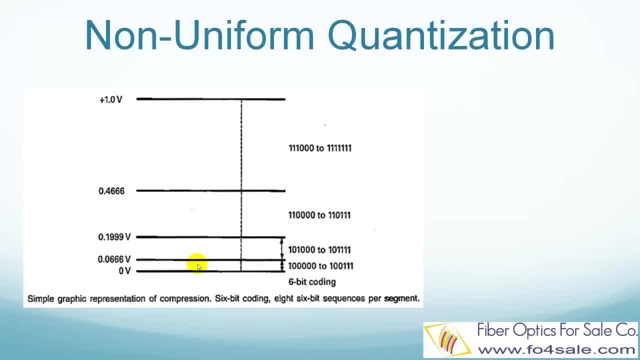 In non-uniform quantization process, the steps are not of equal size. Small steps are used for small signal variation. Large steps are used for large values. The purpose of doing so is to achieve that the signal-to-noise ratio is nearly independent. 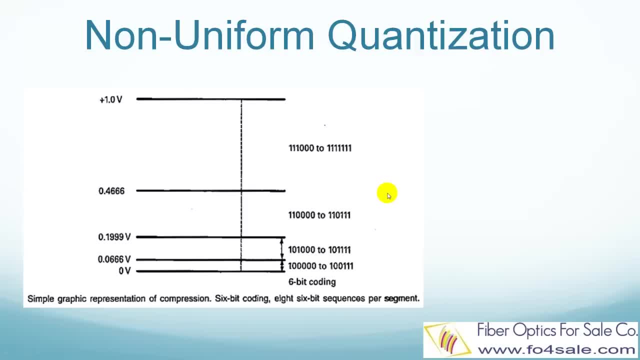 of the signal level. This is done by favoring low-level voice over high-level voice. In other words, more code groups are assigned to speech at low levels than at the higher levels, progressively more as the level reduces. This is shown in this figure. 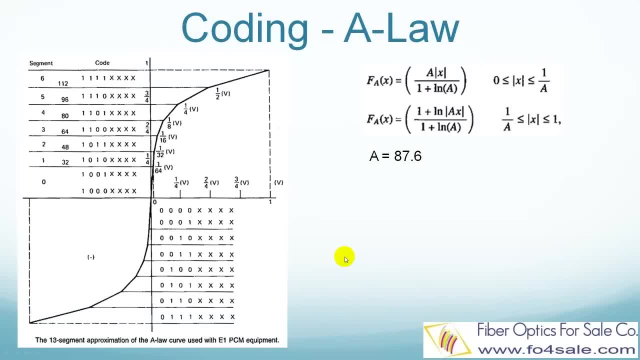 There are two types of non-uniform quantization methods in popular use today. They are the A-Law and the Mu-Law. Let's first look at the A-Law. A-Law follows the logarithmic formula listed here, with A equals to 87.6..